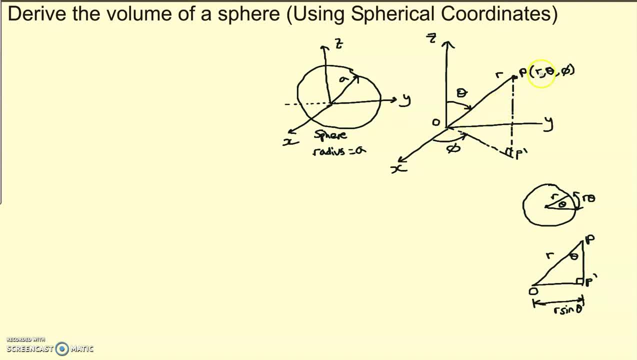 So instead of using x, y, z coordinates, we're going to use r, theta and phi. So r is the distance from the origin to our point in space, And then theta is the angle that the line that connects the origin to p, our point p, makes with the z-axis. 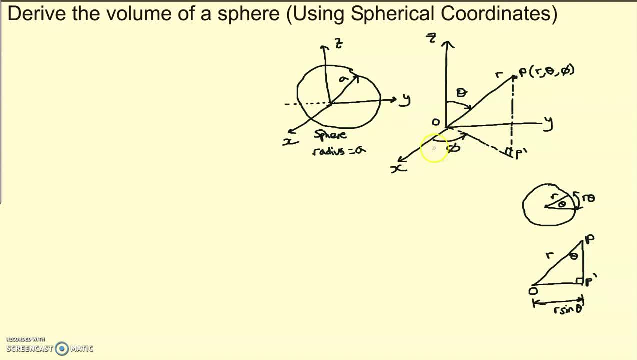 So this is theta, And then phi is the angle that the x-axis This makes with the line that connects the origin to the projection of the point p on the x? y plane. This is p bar. P bar is the projection of our point on the x? y plane. 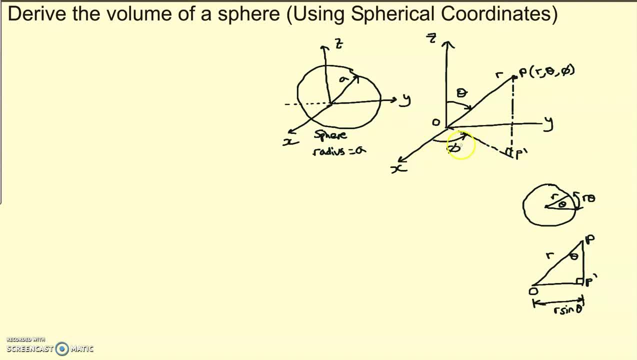 So this angle here is theta is phi. So if we were going to use Cartesian coordinates, then our line elements would have been dx, dy And dz And our volume element would have been the product of these three dx times dy times dz. 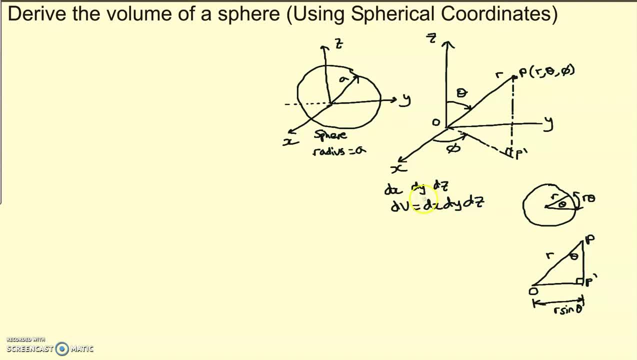 So in spherical coordinates we need to find the three line elements that we're going to use. So for r, for the coordinate r, the line element is just dr For theta. so if you picture here that we increase our angle from theta by a small angle, 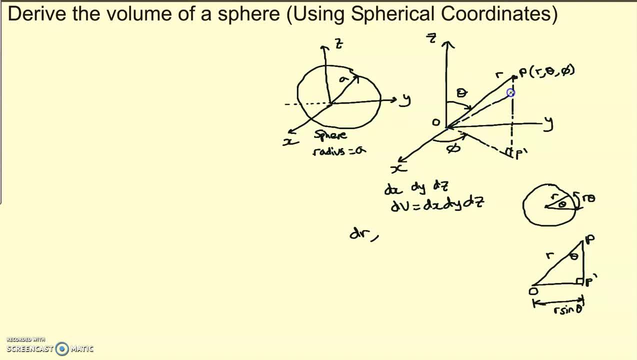 let's call it D theta. So our point p is going to move in space with a small arc here, And let's call this angle d theta. So the point here is going to traverse a small arc And the length of this arc is going to be r times d theta. 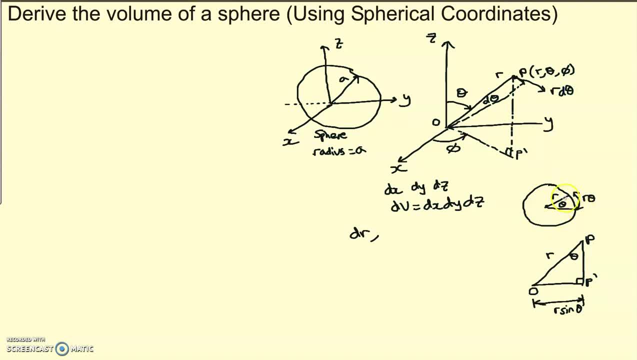 So just a quick reminder: if we have a circle here with radius r and then we have an arc and the angle that subtends that arc is equal to theta, and theta is in radians, then the length of the arc is equal to. 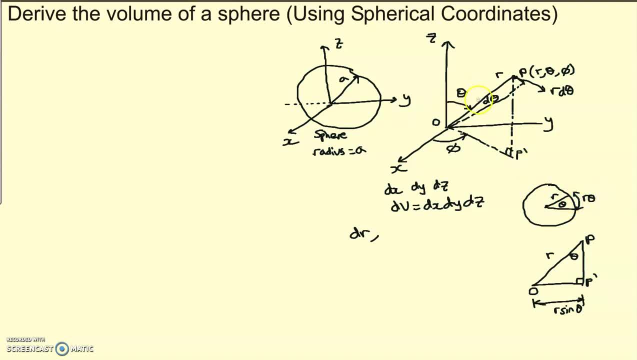 the radius times the angle itself. So this is the same. here We have our small incremental angle d theta And the length of the arc is going to be r times d theta. So that's the line element for the theta component, For the phi component. so if we hold everything else constant, 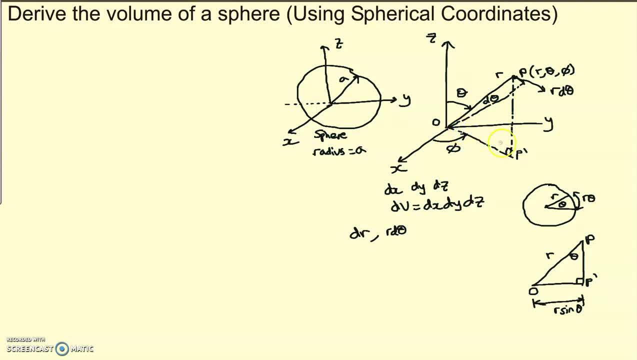 and then we increase phi by a small angle. d phi then the projected point. so if you can imagine that we increase this by a small angle called d phi, then our projected point here is going to traverse a small arc And the length of this arc is going to be the radius. 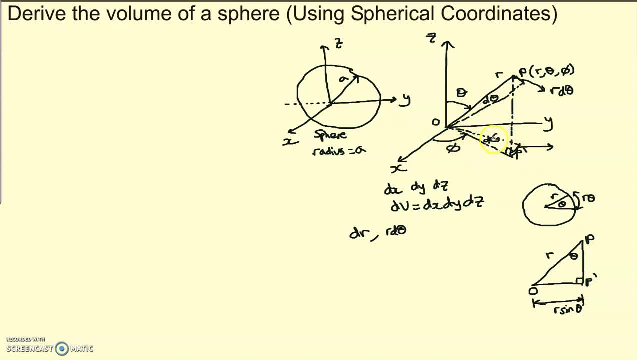 which is this radius here, which is different than r times d phi, And the length of the projection, the length from o to p bar is just r sine theta, And I've drawn that right angle triangle externally. So o is our origin. 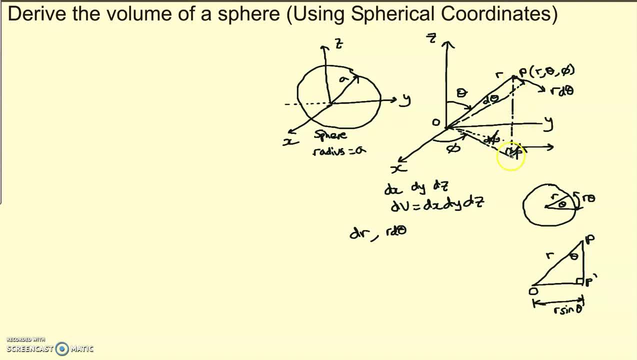 p is our point and then p is the projection And this is a right angle triangle. So if we draw that here we have: r is the length from o to p, p is our projection, The angle that this angle here is theta. 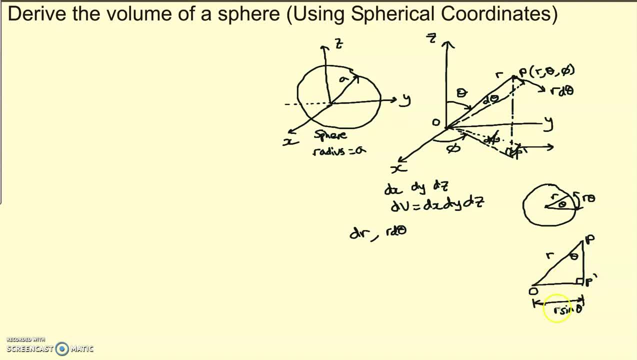 And so the length from o to our projection is just r sine theta. So our line element here has a length of r times sine theta d phi. So that is our third line element. So it's r sine theta d phi. So our volume element. 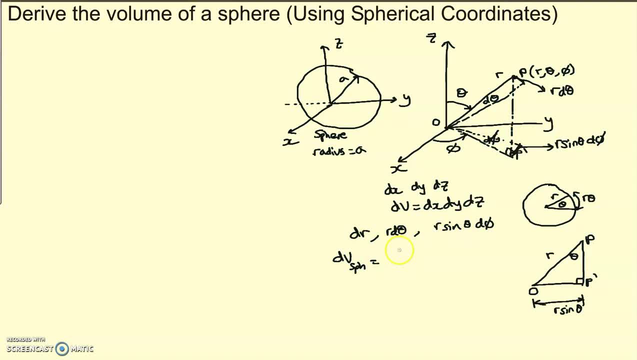 this is in spherical coordinates- is going to be the product of these three, which is r squared sine theta dr, d theta d phi, So the volume of our sphere. so volume is going to be the integral of dv, So it's going to be the triple integral of. 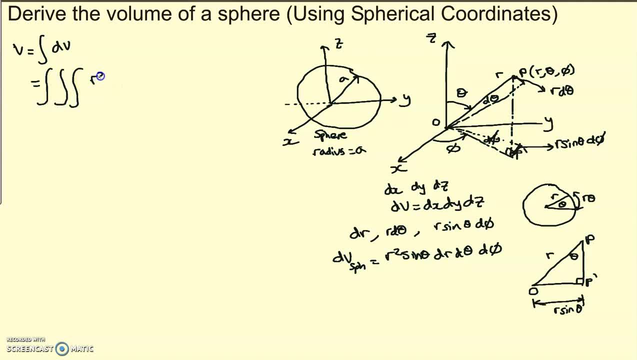 r squared sine theta dr d, theta d phi. And now we need to find the limits of our integral. So if we have a volume element inside of our sphere, let's call this dv. So we need to find the limits of our integral. 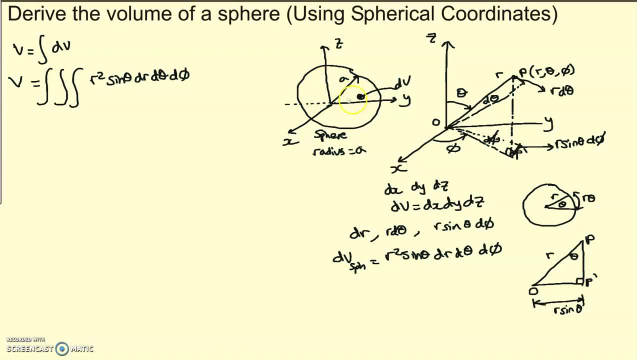 So we need to be able to move this volume element all over the sphere in order to compute the entire volume. So to do that, the volume element needs to move first of all from the center of the sphere all the way to the edge of the sphere. 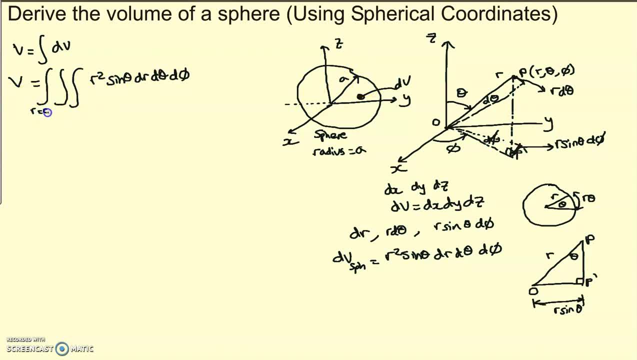 So when we integrate over r, the integral has to be from r equals zero, all the way up to the radius, which is equal to a. How about phi? Well, if we have a volume element, that's here and we're trying to scan through. 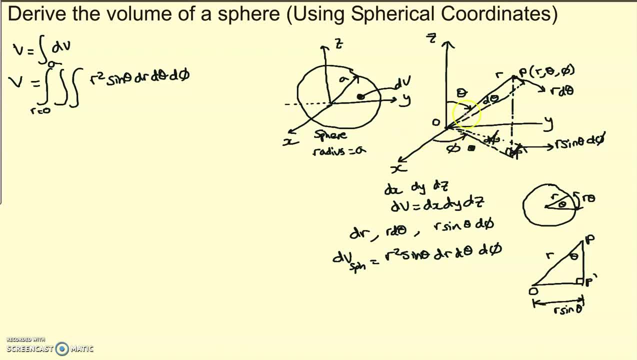 the entire volume of the sphere. then we need to rotate our element all the way all through the entire 360 degrees. So phi needs to be from zero to two pi, So to cover the entire 360 degrees. Now for our angle, theta. 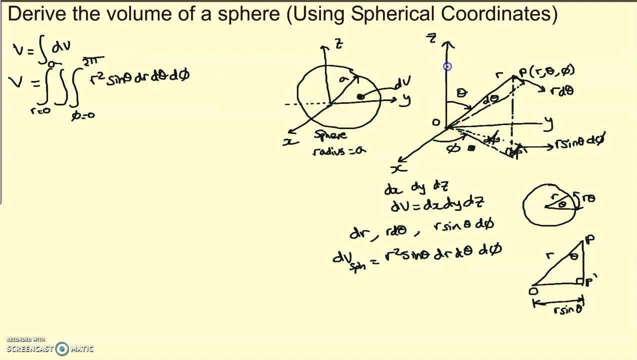 theta equals zero is going to be when, let's say, our element here is aligned with the z-axis and it needs to go from zero all the way to the other side, which is going to be from zero to pi. So our angle here: 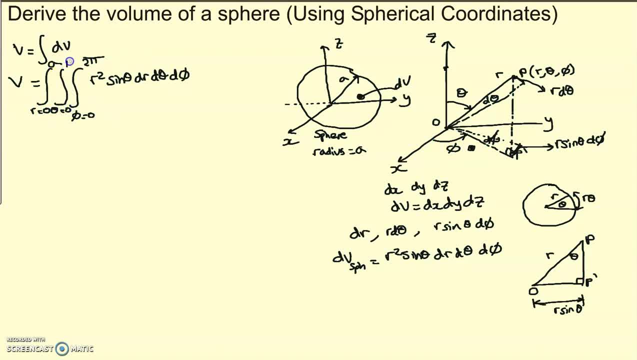 theta is going to be equal to zero all the way to pi. not two pi, just pi. So, even though this is a triple integral- but it's actually a very simple one- There's no dependency among the three integrals. All three are independent. 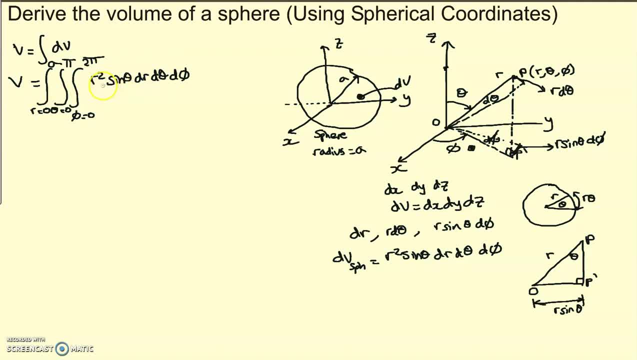 So we actually can split this triple integral into three separate integrals. So we have the first integral from r equals zero to a of r squared dr, And then the second integral is going to be from theta equals zero to pi of sine theta d theta. 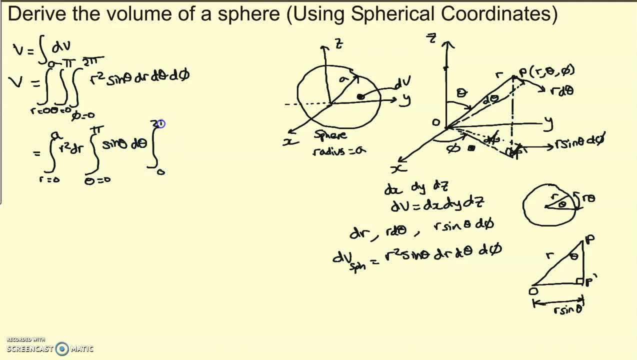 And the last integral is going to be from zero to two pi of d phi. So the first integral of r squared is going to be r cubed divided by three, And the limits of the integration is going to be from zero to a. The second, 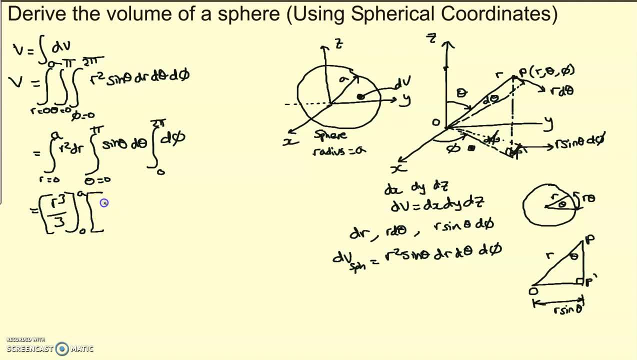 integral. integral of sine theta is going to be minus sine theta, but i'm going to write it as cosine theta and instead of putting pi and zero, i'm going to flip the order here so it becomes zero and pi. so i flip the order because the integral of sine theta is negative cosine theta.